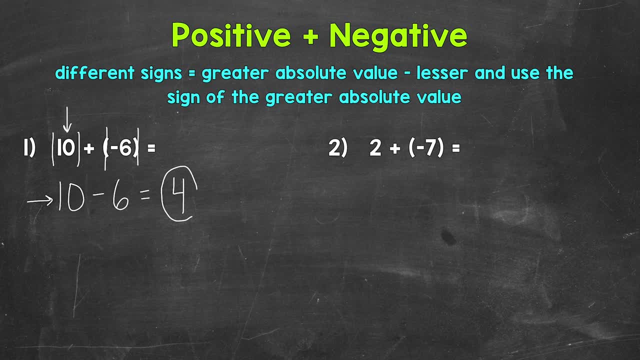 our original problem. So we're going to take the sign of the larger absolute value and subtract the lesser, So our answer is going to be a positive 4.. Our final answer: positive 4. Basically, we forget about any negatives because we are working with absolute values. Find the difference. 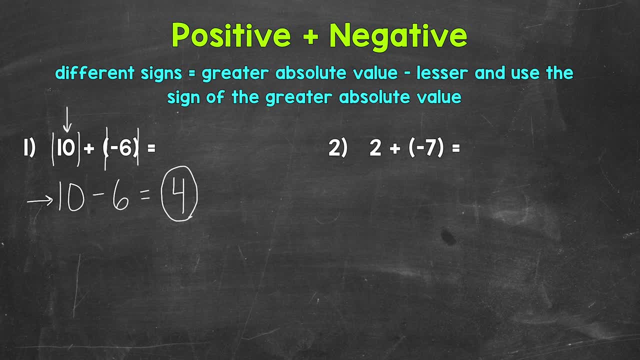 between absolute values and then take the sign of the greater absolute value from the original problem. Now let's think through this a second way, And this way is going to be more of a mental math approach: Just basically thinking about the greater absolute value and subtracting the lesser. 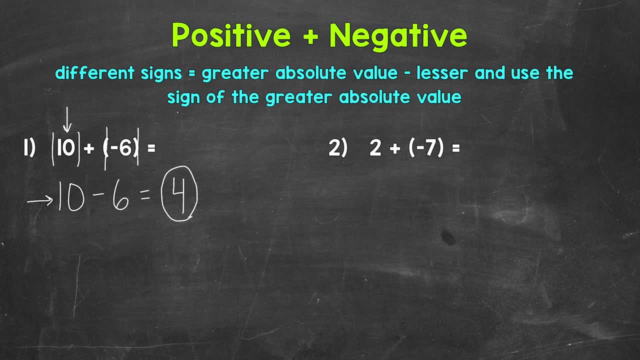 Now let's think through this a second way, And this way is going to be more of a mental math approach- Just basically thinking about what's going on in this problem. I'll rewrite the problem down below. So we have 10 plus negative 6.. So let's think about this. So we are starting at a positive. 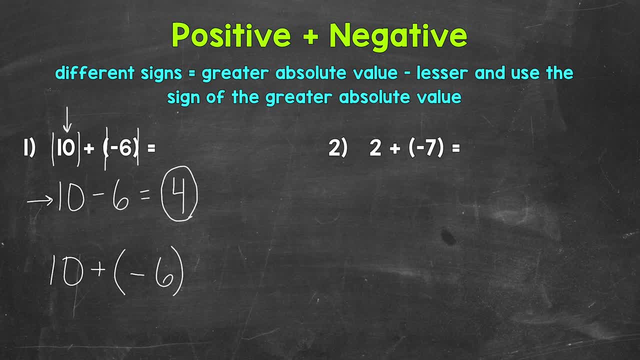 10 and we are adding a negative 6.. By adding a negative 6, we are decreasing in value by 6 from that 10.. We can basically think of this as 10 minus 6, or 10 take away 6. That gives us our answer of 4.. So 10 plus negative 6 gives us. 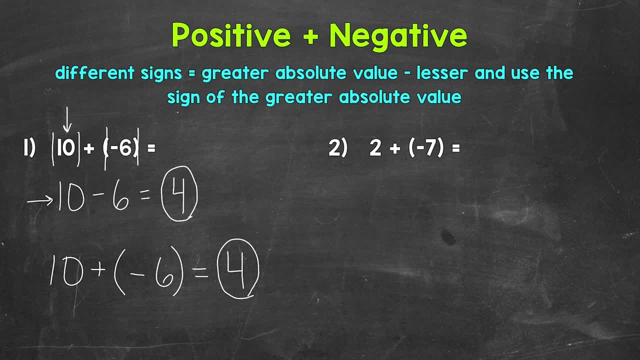 4.. So again we started at positive 10.. Always think about where you are starting and where you are going from that starting point. So we are adding a negative 6, which is decreasing our 10 in value by 6. And we end up with a negative 6.. So we are adding a negative 6,, which is decreasing 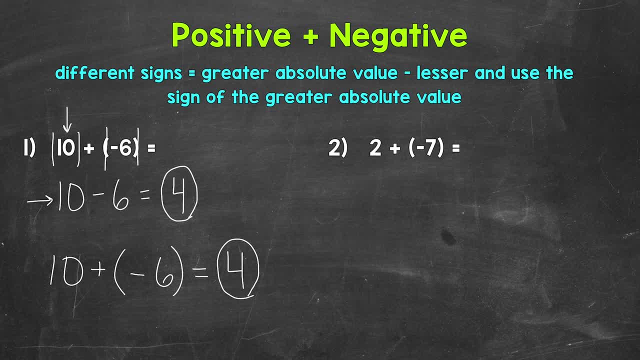 our 10 in value by 6. And we end up with positive 4 for our final answer. Let's move on to number 2, where we have 2 plus negative 7. So we have different signs here, a positive and a negative. So we take the greater absolute value and subtract the lesser We use. 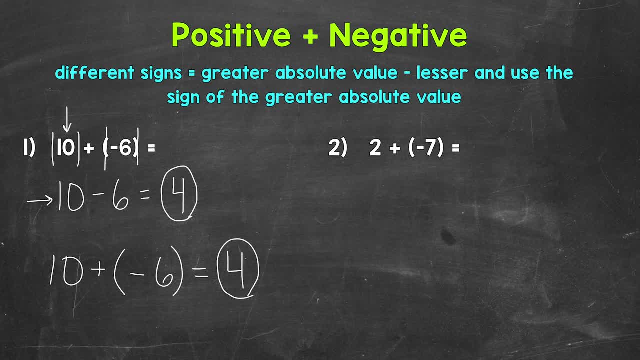 the sign of the greater absolute value for our answer. So let's take the absolute value of 2,, and that is going to be 2.. And then the absolute value of negative 7, is 7.. So we have 2 and 7 there. We need to take the greater absolute value and subtract the lesser.